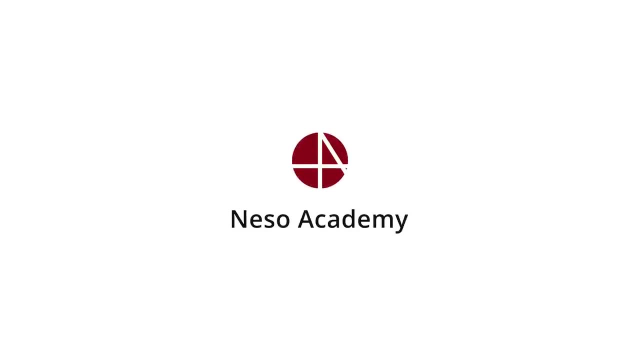 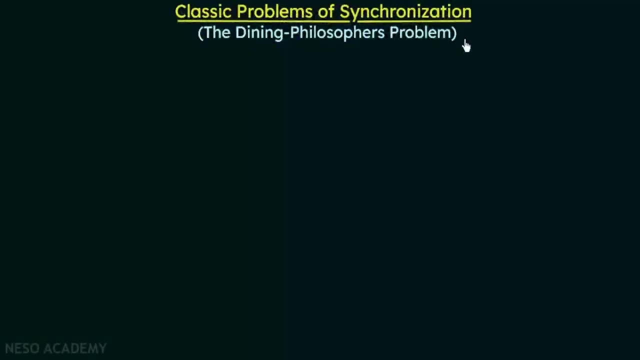 In this lecture we'll be discussing about another classic problem of synchronization, which is known as the dining philosopher's problem. So first of all, we'll be trying to understand what is this dining philosopher's problem, and then we'll be seeing if we can solve. 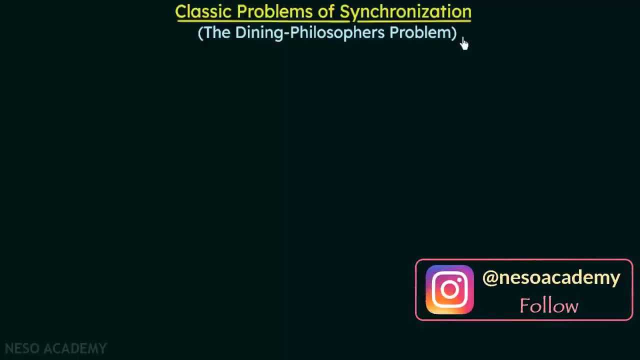 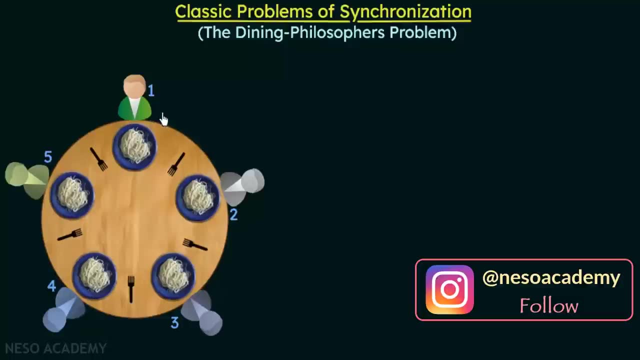 this using semaphores, Alright. so first let's see: what is this dining philosopher's problem? So in this dining philosopher's problem, what we have is we have a round dining table in which we have, let's say, five philosophers who are seated around the table like this. So the philosophers. 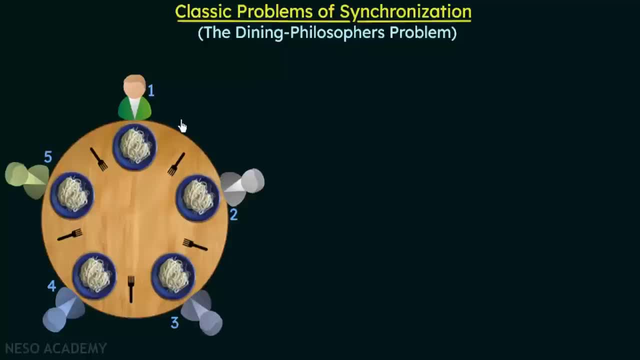 here they can be in two states, which is the thinking state and the eating state. So the philosophers: here they spend their whole life either thinking or eating. So when the philosophers are thinking they don't interact with their colleagues, here They just mind their own business. 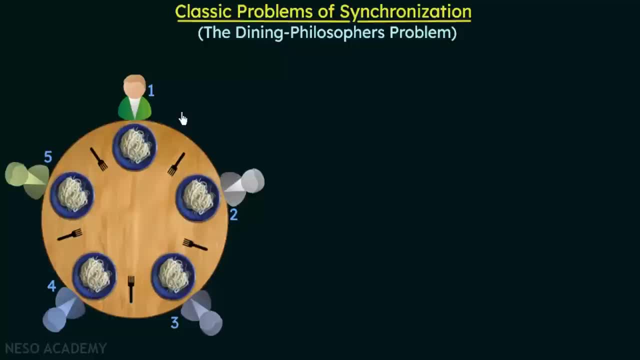 and they think: And when they are hungry, they will try to eat this rice or noodles that are present in the plate that is present. So when they are hungry, they will try to eat this rice or noodles that are placed before them. Now the thing is, when the philosopher wants to eat the 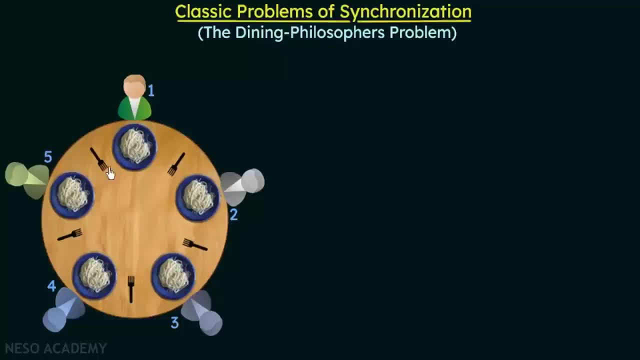 food that is placed in front of them. they need to make use of these forks or the chopsticks that are there, that are placed adjacent to them. So when a philosopher wants to eat, he needs to make use of two forks or two chopsticks that are placed here. They cannot eat with just one, but they need. 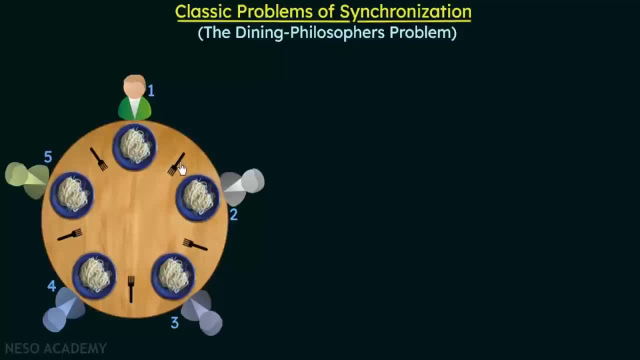 two of them. So when a philosopher gets hungry, he will take up the two forks or chopsticks that are adjacent to him at his right hand side. So when a philosopher wants to eat, he needs to eat with his left hand side and then he can start eating. So when he starts eating, nobody can. 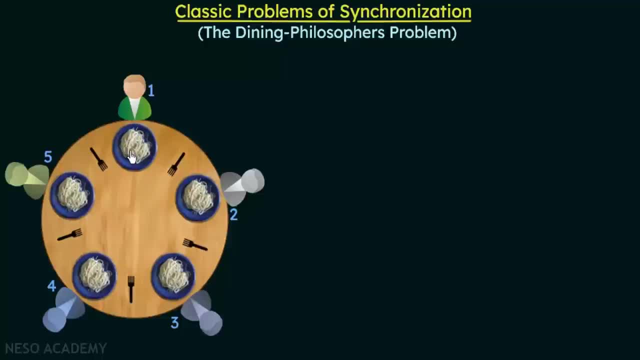 disturb him or nobody can take the fork away from him, And then when he finishes eating, he will be placing the forks or chopsticks back at their places. So what is the problem here? So if you look at this diagram carefully, we can see that the chopsticks or the forks are limited. There are 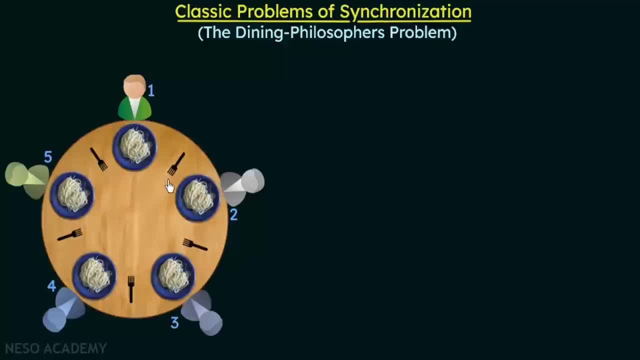 five philosophers, and how many forks are there? One, two, three, four, five? There are only five forks and I think that the forks are limited. So when a philosopher wants to eat, he needs to make use of two forks or two chopsticks. So clearly we see that it is limited, Like for. 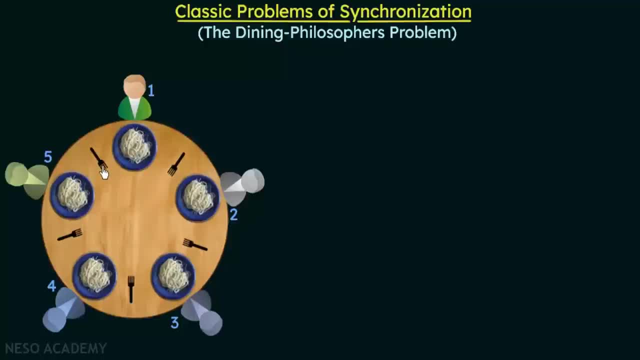 example, when philosopher one will want to eat, he will make use of this and this fork And, at the same time, if philosopher two gets hungry, this philosopher two needs to make use of this fork and this fork, But we see that this fork is being used by philosopher one, So he will not be able. 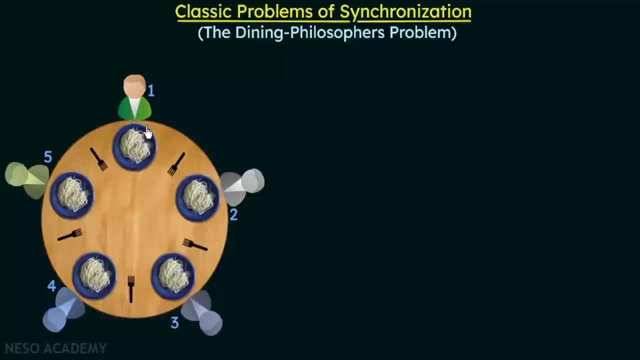 to eat when philosopher one is using the fork that is adjacent to him. So we have to make sure that no two philosophers that are adjacent to each other try to eat at the same time. So if they try to eat at the same time, we are going to have a problem. So, as I told you, 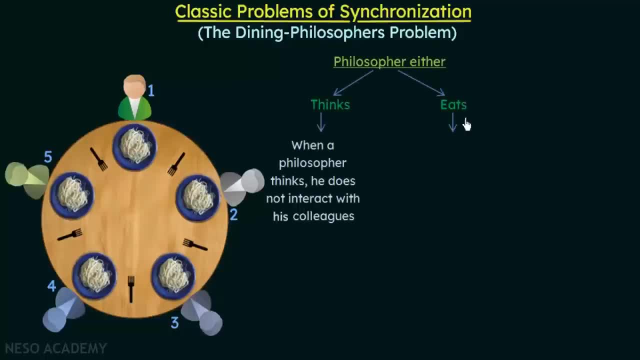 the philosophers can be in two states: the thinking state or the eating state. So when a philosopher is thinking, he does not interact with his colleagues, He just minds his own business and he thinks and he does not disturb anyone. And now when he eats, what happens When a philosopher 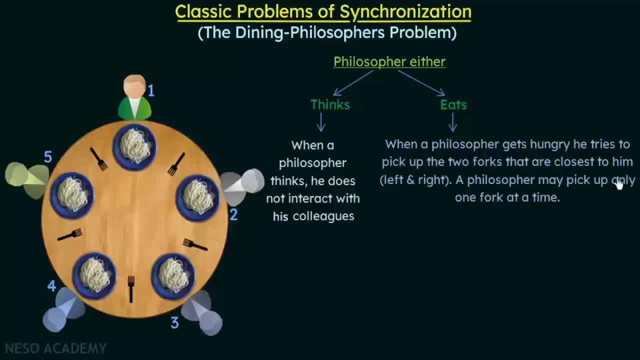 gets hungry, he tries to pick up the two forks that are close to him and he tries to eat them, So he loses to him left and right. A philosopher may pick up only one fork at a time, So this is also an important thing. He needs two forks for eating, but also he cannot pick up both the forks at the 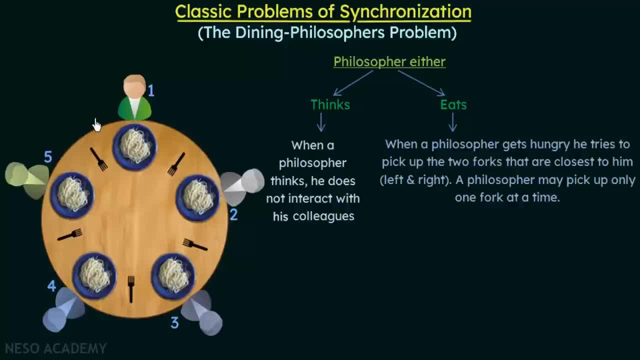 same time He will have to pick up one fork and then after that he will have to pick up the other fork. So that is also an important thing that we need to keep in mind in this problem. And also, one cannot pick up a fork that is already in the hand of a neighbor. So that also I have already. 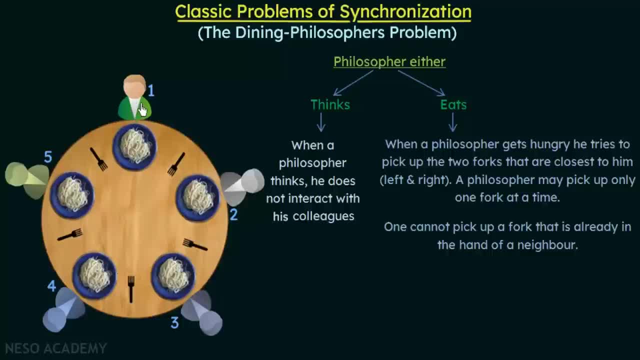 shown here, When a fork is being used by one of his colleagues, he will have to pick up one fork: the philosopher. no other philosophers can use that particular fork. So I told you like when philosopher 1 is eating, he'll be making use of this fork and this fork which are at his right. 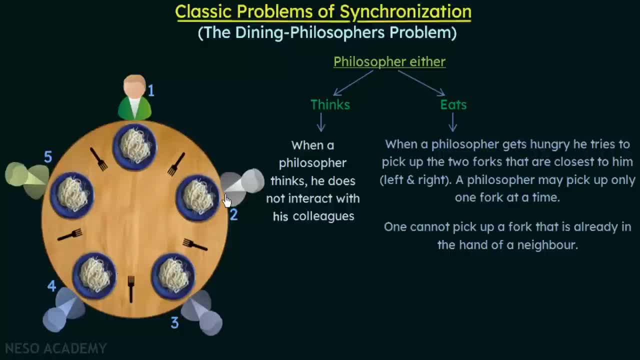 and left. So at the same time, if philosopher 2 tries to eat, he also needs to make use of this fork and this fork, But this one is held by philosopher 1.. So 2 will not be able to eat. 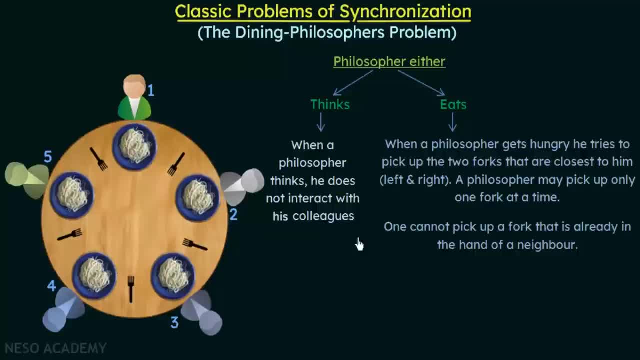 because he will not be able to get hold of this when 1 is eating. So that is what we mean here. And then, when a hungry philosopher has both his forks at the same time, he eats without releasing his forks. When he has finished eating, he puts down both of his forks and starts thinking again. 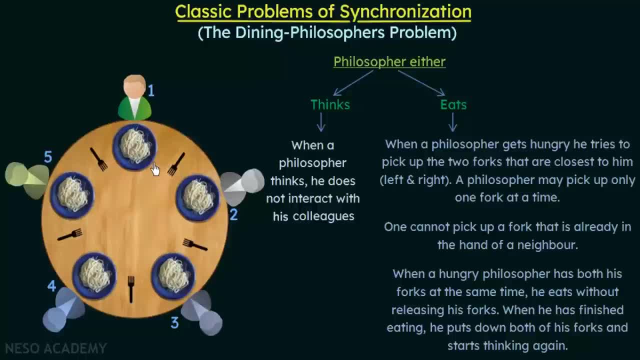 So when a hungry philosopher gets hold of both the forks, he will be eating and after he completes eating he will be placing the forks back where they were and then he will start thinking again. So this is the scenario that we have in a dining philosopher's problem. 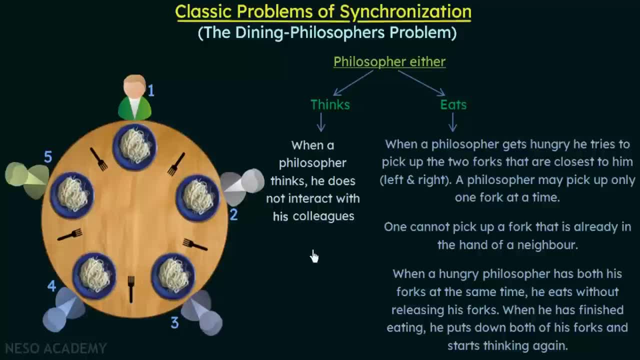 So what is the actual problem here? I have already told you: The problem is that, since the forks are limited, no two adjacent philosophers should be allowed to eat at the same time, So no two philosophers should try to access the same fork at the same time. So that is the problem that we have. 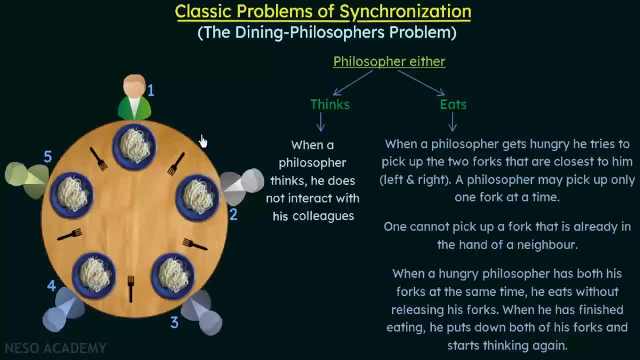 here. Okay, so now you may be thinking: why are we discussing about this dining philosopher problem, Why are we creating a story like this and why are we trying to solve this problem? So, if you think about it, this is actually a problem of: 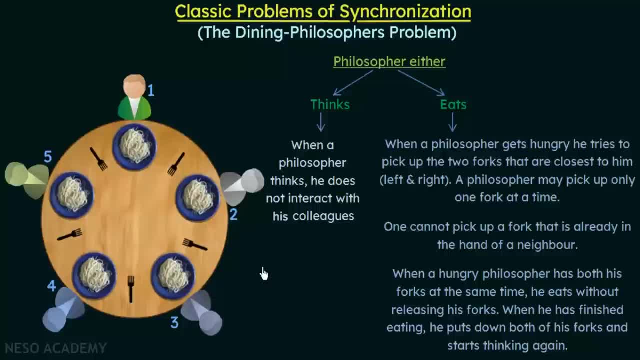 operating philosophy. Why are we creating a story like this and why are we trying to solve this problem? Okay, so this should be directly worrying justification. The rule of law is to take the same skill- friends playing around with things as their master, and then just 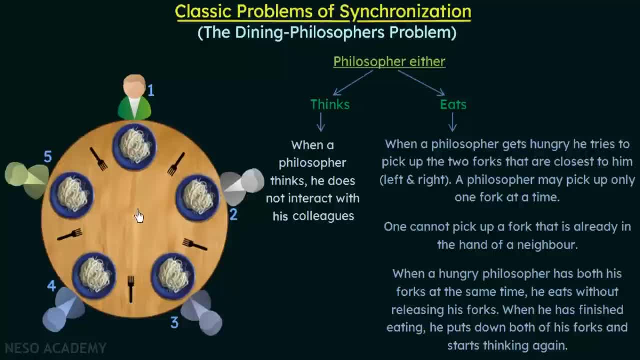 devise new rules and daily rules between such a class and for such a class before the mentor is be late in the class, So before the mentor has seen the life-inguémure, the mentor will have a cast-on lecture where he or she will tell the student on Fa-D��서. 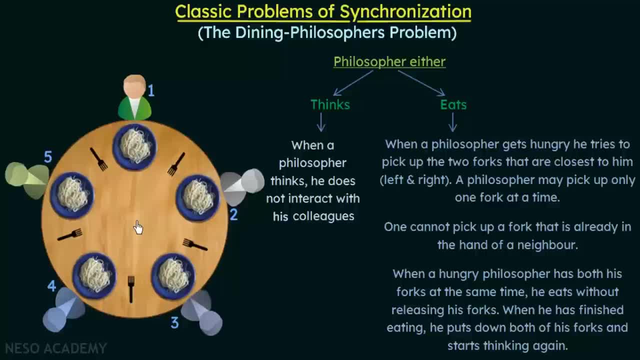 that once he is completed with fa-Dosa, the teacher is removed from the class and thus will be independently practicing Fa-Dosa on the first and last day. So in the course of the lecture, if neither of the teachers have taken the proper training to solve the problem, 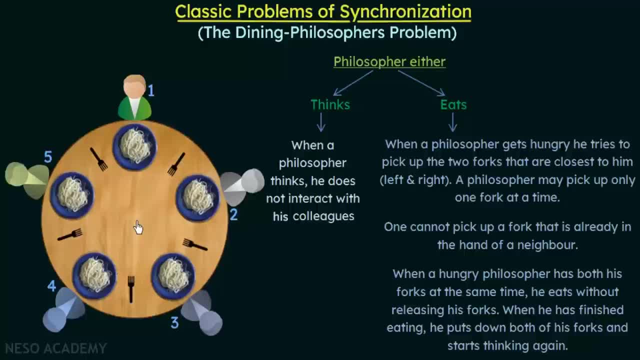 at the same time, then we will be having problems in the operating system. So that is why we are discussing about this Dining Philosophers problem. It is actually a problem of resource allocation and how the resources are being utilized when they have to be shared. 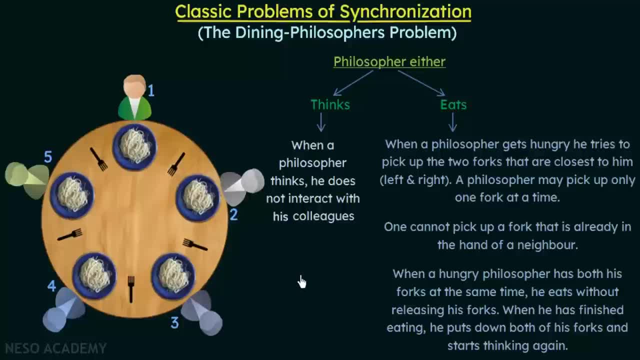 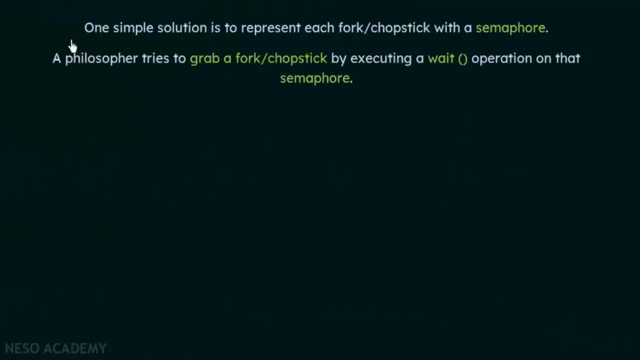 among processors. Alright, so now we have understood the problem statement of this Dining Philosophers problem, and now we will be seeing how can we solve this using semaphores. So one simple solution is to represent each fork or chopstick with a semaphore. 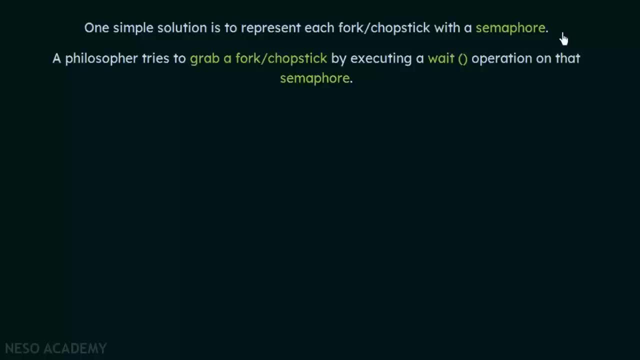 So we know that a chopstick or a fork should be used by only one philosopher at a time, and when one philosopher is holding it, no other philosopher should be allowed to take it away from him and he should not allowed to access that same fork at the 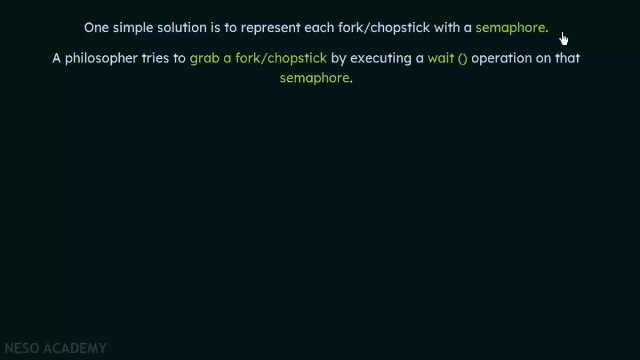 same time. So we can do that with the help of semaphores. So a philosopher tries to grab a fork or chopstick by executing a wait operation on that semaphore. So now what we will be doing is we will be representing each of these. 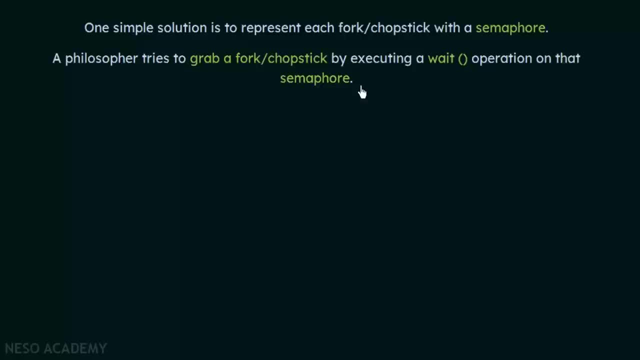 forks or chopsticks with the help of a semaphore. So we already know the features of semaphore and how they work. So when a philosopher wants to grab a fork or chopstick, he will be executing a wait operation on the semaphore or the chopstick. So we know what happens. 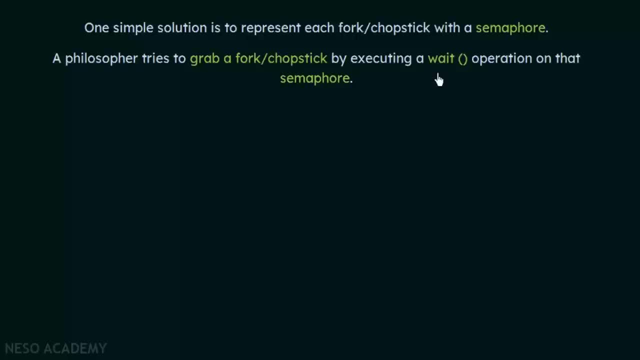 when a wait operation is executed on a semaphore. So when a wait is executed, it implies that that particular process wants to use that semaphore and it wants to get hold of it, and when it gets hold of it no other processes will be allowed. 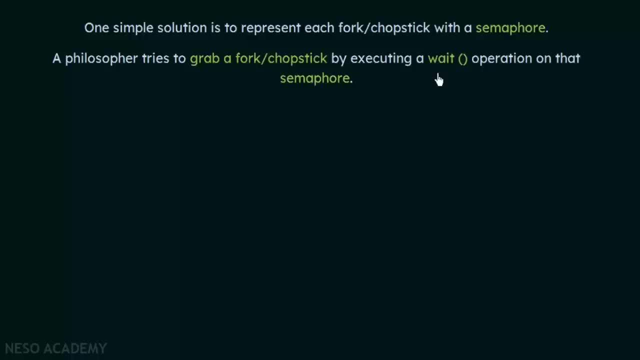 to use that semaphore. So, similarly, we will be applying this on the chopsticks or the forks that we have here. So the philosopher will execute a wait operation on the chopstick when he wants to use it, And then he releases his fork or chopstick. 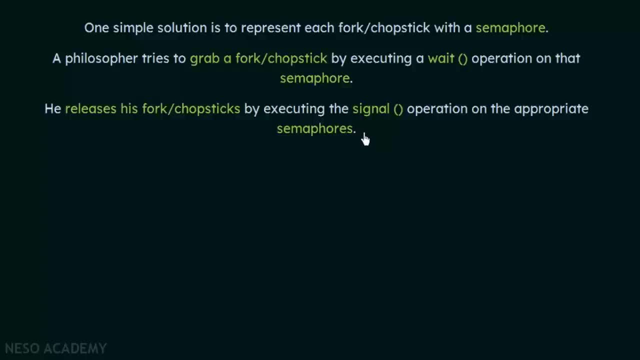 by executing the signal operation on the appropriate semaphores. So after the philosopher finished eating, he will have to put back the chopsticks or the forks at their places. So at that time, how will he do? He will be doing. 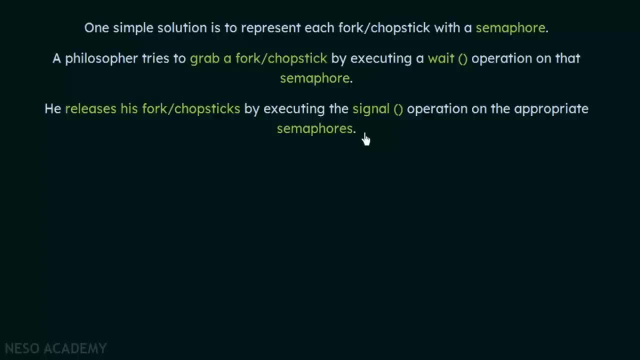 so by executing the signal operation on the chopstick or the fork, because we are assuming that they are semaphores. So when a signal operation is executed, what happens? We have already studied that in semaphores, signal operation means we are releasing. 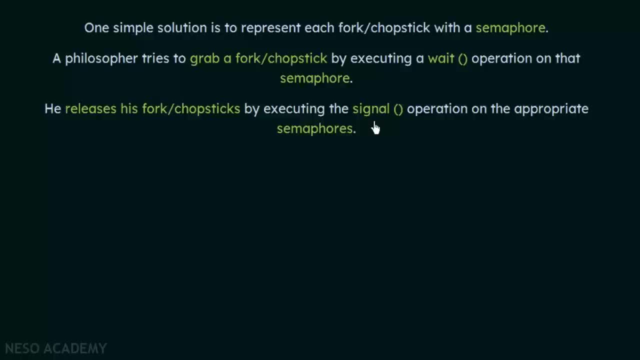 it. So a philosopher will be releasing his fork or chopstick by executing the signal operation. So how we will be implementing this is we are having five chopsticks or five forks. We have seen that in the diagram. So each of these, 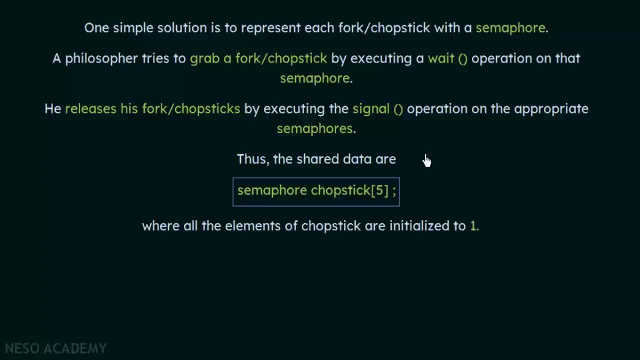 chopsticks will be represented as a semaphore. So what we are doing is we are having an array of chopsticks with the data type semaphore, So the data type is semaphore, and we have five number of chopsticks, So we are using an array. So what we mean 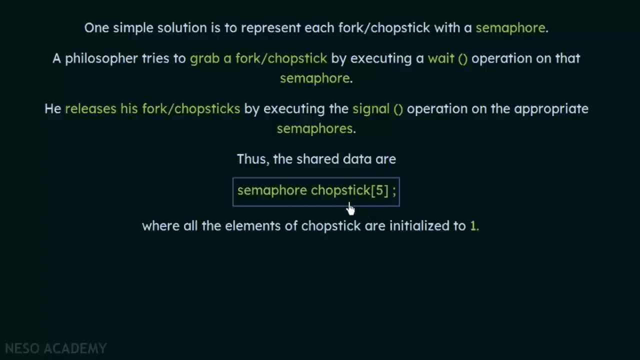 by this chopstick five is that we are having an array of five elements. So we will be having chopstick one, chopstick two, chopstick three, chopstick four and chopstick five. So these are the five chopsticks we have, and they are. 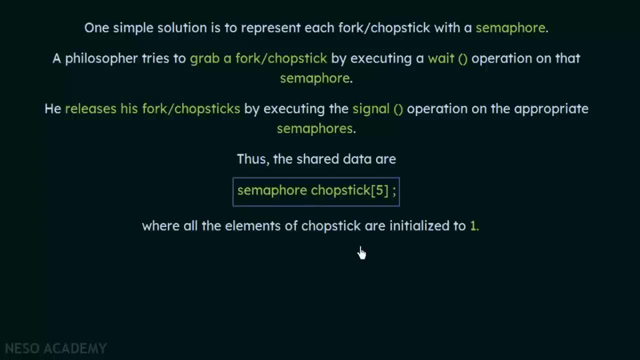 all declared as semaphores And here all the elements of the are initialized to 1.. So here the semaphore that we are going to use is a binary semaphore, not a counting semaphore, but a binary semaphore, And we know that in binary semaphore it can take. 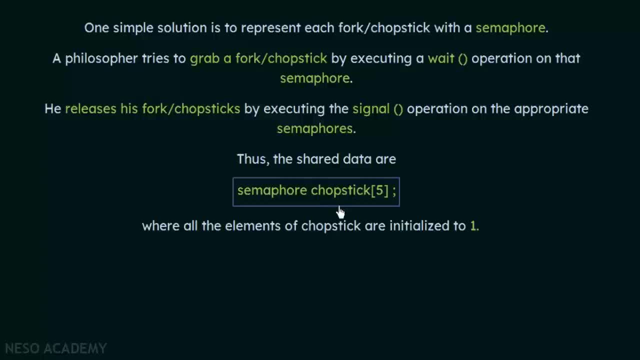 two values, either 1 or 0. So don't confuse this with a counting semaphore. here Chopstick 5 actually means it's an array of chopsticks that we are having: Chopstick 1,, 2,, 3,, 4 and 5.. 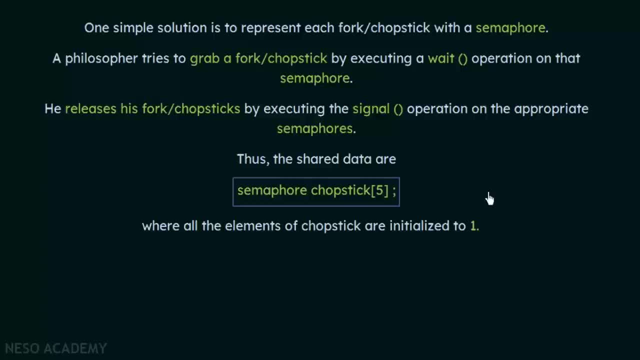 And each of these chopsticks can have two values, either 0 or 1.. So initially all the elements of the chopsticks are initialized to 1.. So in a binary semaphore, when it is initialized to, 1 means it is free. 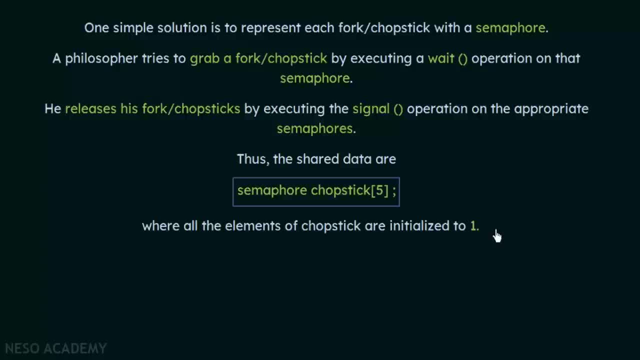 It can be used by the processors that wants to use it, And if the value is 0, that means it is currently being held by some processors. It is not free, So that is what we mean here. So all the chopsticks will be initialized to. 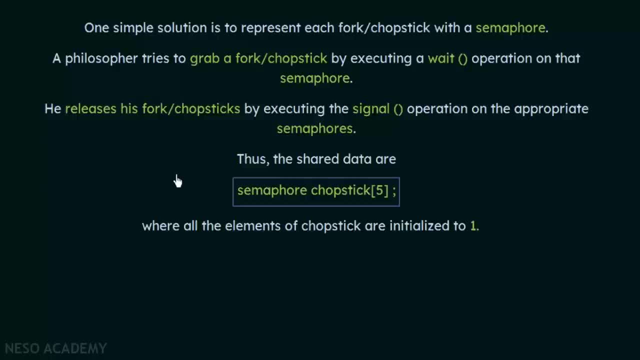 one initiative, Alright. so this is how we are going to make use of the semaphores to solve this problem. So now we will be seeing the structure of the philosopher. That means we will be seeing how the code is written in order to accomplish this. 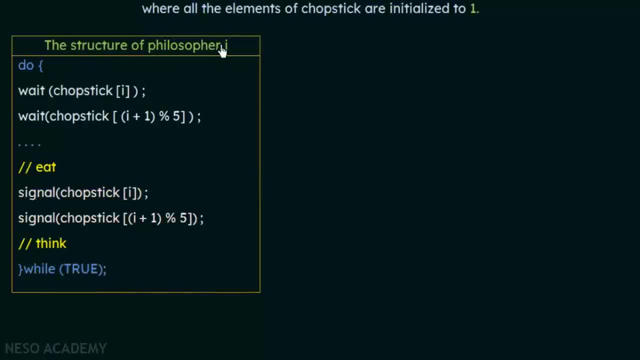 So here is the code. This is the structure of any philosopher. I Here what will happen When a philosopher wants to eat his food. that means, when he is hungry and when he wants to eat, what is the first thing that he needs to do? 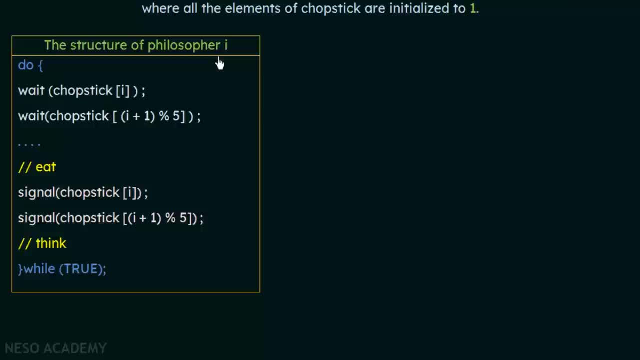 He needs to get hold of the two chopsticks that are adjacent to him. So he needs to get the chopstick at his left and right. How will he do that? So, as I told you, we are going to assume that these chopsticks are semaphores. 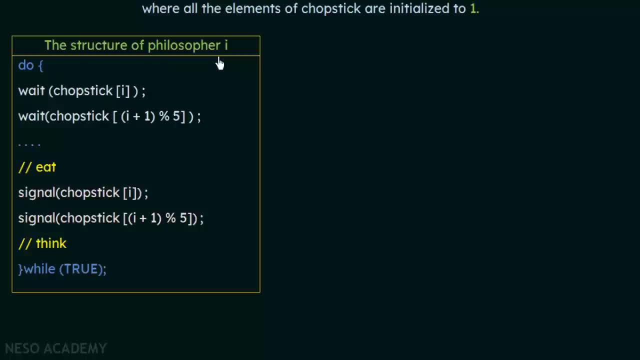 So he will have to execute a weight operation on two forks or chopsticks that are adjacent to him. So for philosopher I he needs to execute a weight operation on chopstick number I and then also on the chopstick I plus one modulo. 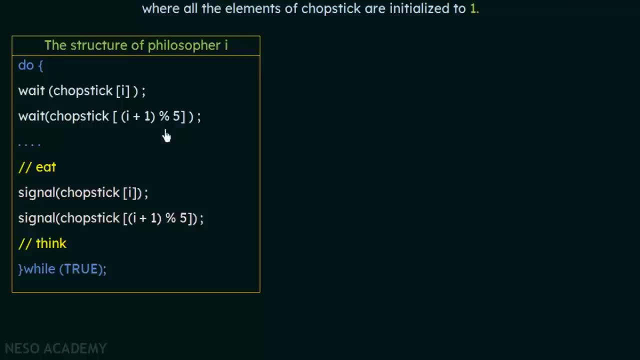 five. So why we are making use of this mod five is because, as I told you, the philosopher will need to access the two forks that are adjacent to him, So let's say that we are talking about philosopher one. So 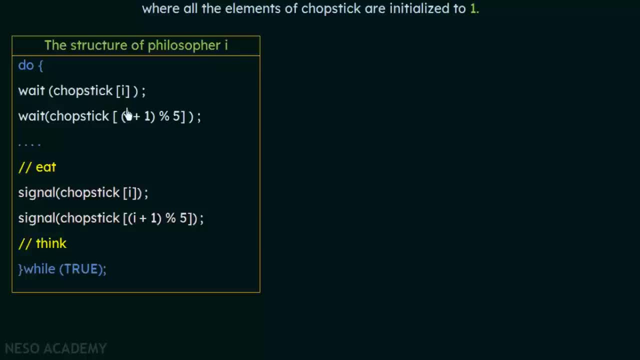 he will need to access fork number one and fork number two. So chopstick I will mean chopstick or fork number one, and chopstick I plus one will mean chopstick number two. So this calculation will be going on, but think of the scenario when we reach. 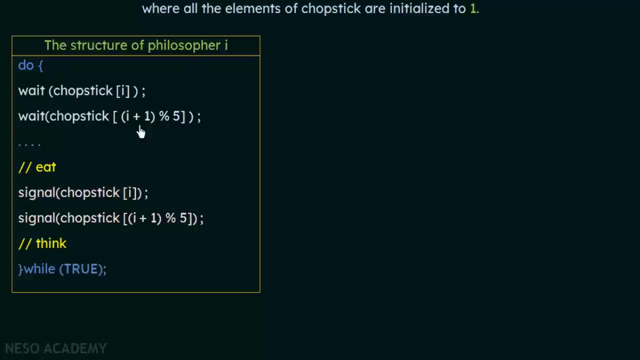 the fifth philosopher. So the fifth philosopher will need to make use of which chopstick? He will make use of chopstick number five. So if we just write here I plus one, then what happens? Five plus one will give us six, which means chopstick number. 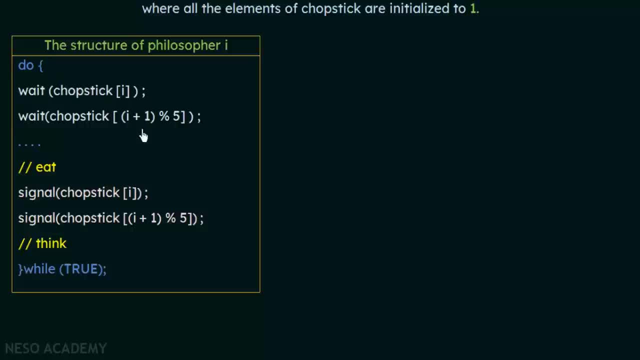 six. but there is no chopstick number six, So after the chopstick number five it has to make use of chopstick number one again. It is placed in a circular fashion, So it goes like one, two, three, four, five Again. 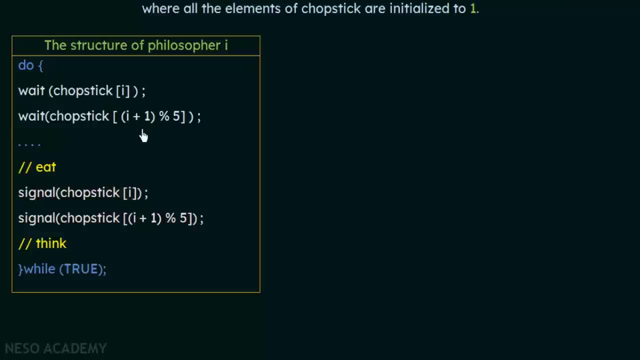 one, two, three, four, five. So philosopher number five will need to make use of chopstick five and chopstick one. So that is why we are making use of this mod five here. So, for example, when we reach the fifth chopstick, what will happen? 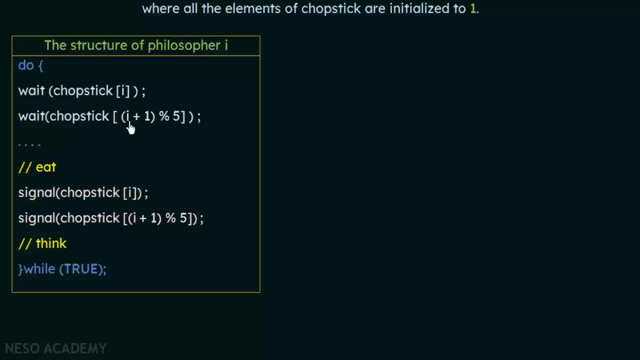 Here it will be chopstick number five. I is equal to five, and here we will have five plus one equal to six, and six modulo five will give us one. So we will get chopstick five and chopstick one. So that is why this calculation is done. 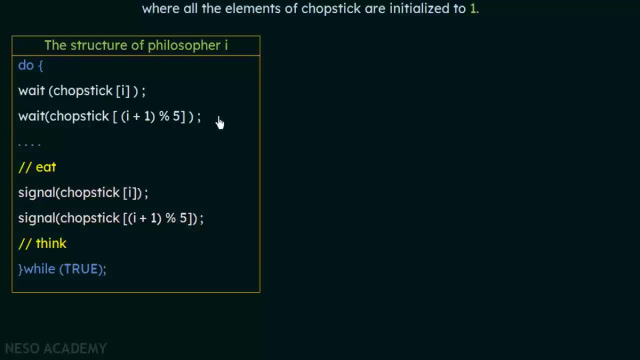 So this is just a pseudo code. When you will be writing the real code for this, you have to carefully design this one, Okay, So what basically it means is that the philosopher needs to execute weight operation on the two adjacent chopsticks that are: 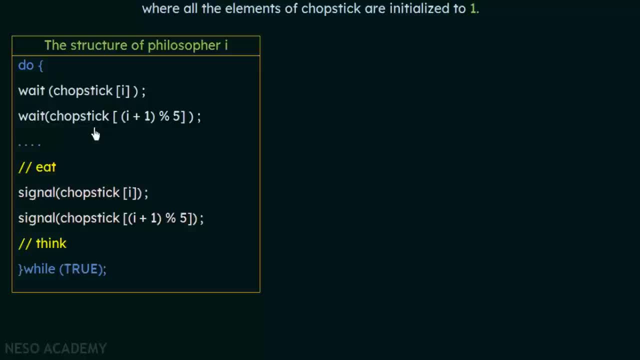 placed near him. Okay, Once he executes these weight operations, if these chopsticks are available, he will be getting hold of them one by one, And once he has hold of both of them, then he can begin eating. So he will be doing the eating operation. 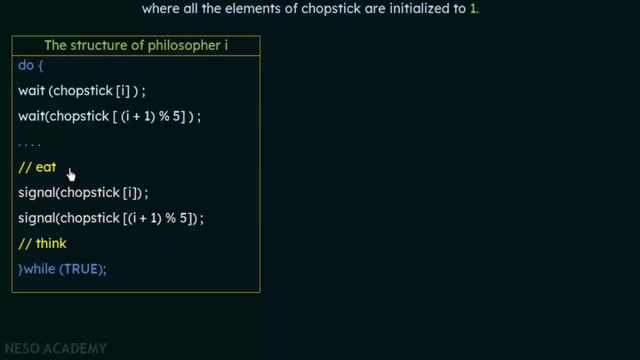 here and after eating, he has to place the chopsticks back where they were so that other philosophers can make use of those chopsticks. So what will he do? He will have to use the signal operation of the chopsticks, So the same chopsticks that he used here. 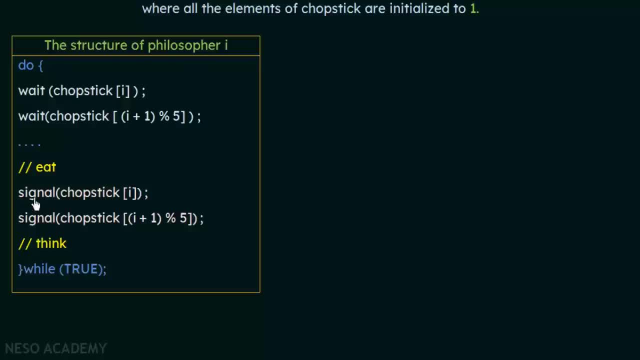 he will be executing the signal operations for those chopsticks. So signal of chopstick i and signal of chopstick i plus one mod five, So that means he has released the chopsticks, and then he will start thinking again. So here we see that when 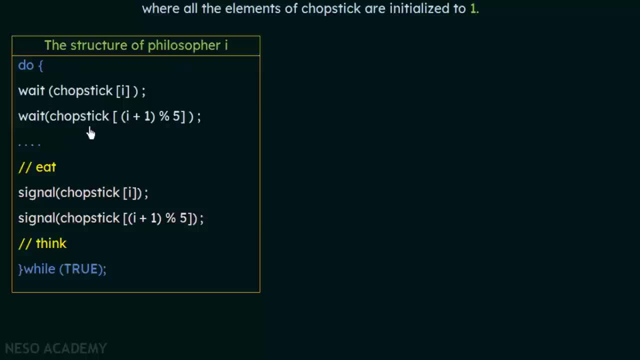 philosopher, i is making use of the two adjacent chopsticks. the philosopher next to him, or the philosopher adjacent to him, tries to also eat. at the same time, he will also try to execute weight on one of these chopsticks, And at that time he will not be able to get it. 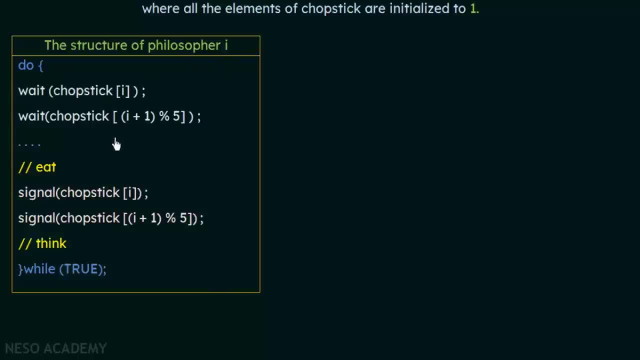 because it is currently being held by this philosopher, i. So we see that two philosophers adjacent to each other will not be able to eat at the same time, and they will not get the same chopsticks at the same time. So, using semaphore, we have solved. 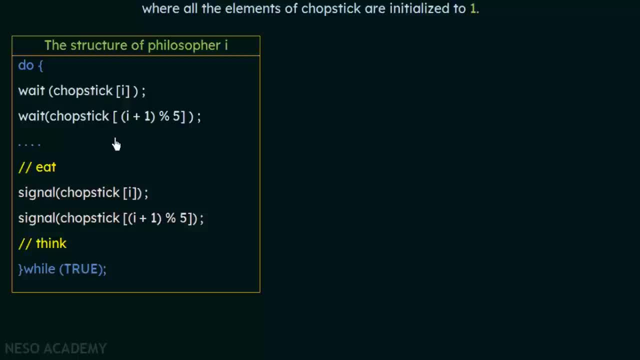 that problem. Okay, So now we have found the solution to that problem. But just by doing this have we solved all the problems? Let's see So here. although the solution guarantees that no two neighbors are eating simultaneously, it could still. 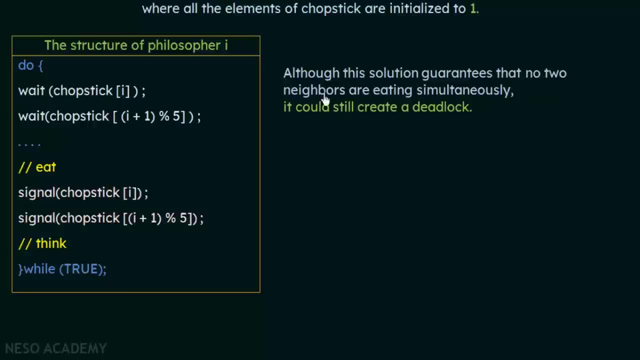 create a deadlock. So we have proved that the solution guarantees that no two neighbors are eating simultaneously. We have already explained that, But this could still create a deadlock. And how is that Suppose that all five philosophers become hungry simultaneously and each grab? 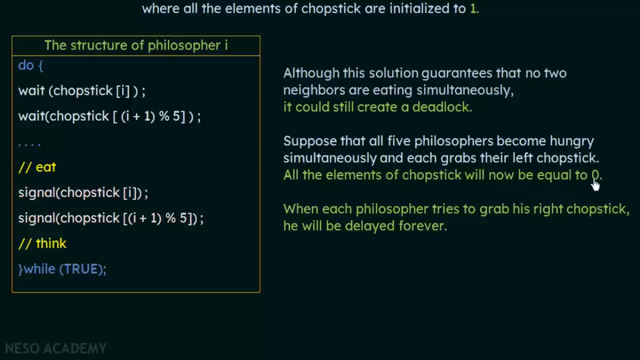 their left chopstick. All the elements of chopstick will now be equal to zero. When each philosopher tries to grab his right chopstick, he will be delayed forever. So think of a scenario when all the philosophers get hungry at the same time. 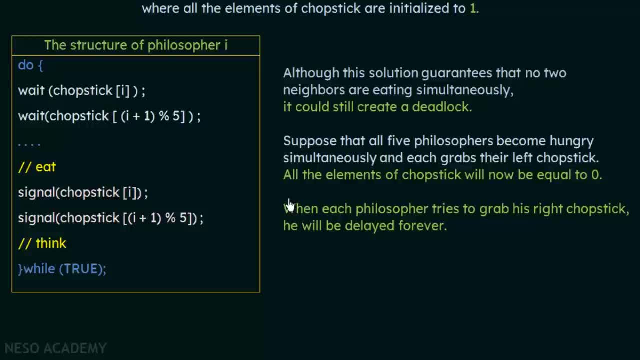 So what will they do? They will simultaneously grab their left chopsticks. So let's say that all of them have grabbed their left chopsticks. Now what will happen? All the elements of chopsticks will be now equal to zero. 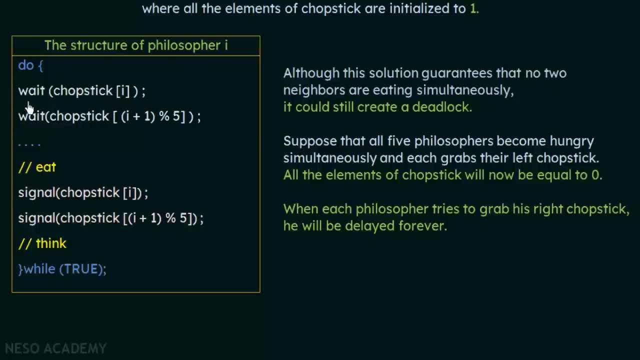 So whenever a philosopher will grab his chopstick, he will execute a wait operation on that chopstick. So when he executes a wait operation, the chopstick's value, which is a semaphore- will be changed from one to zero. Initially they were all one. They will be. 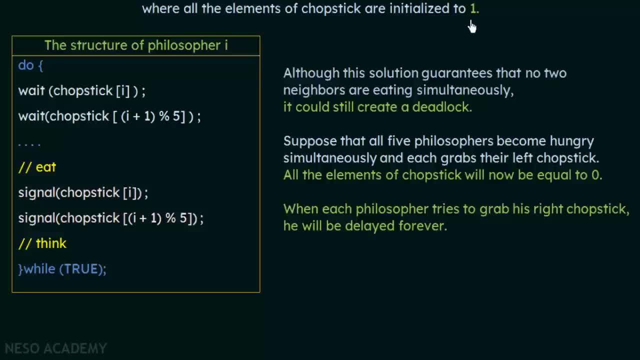 changed to zero, which means that it is now being held by a particular philosopher. So now, when each philosopher tries to grab his right chopstick, he will be delayed forever. So let's look at the diagram and understand this. So here the scenario that we are talking about. 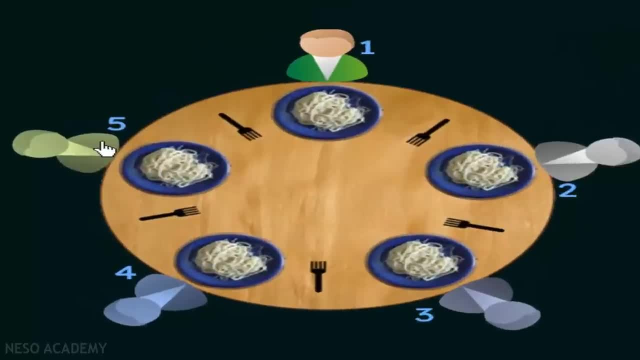 is, all the philosophers get hungry at the same time. And what happens? Let's say that all of them will grab their left chopsticks at the same time. So we already explained that they can not pick up both the forks at the same time. 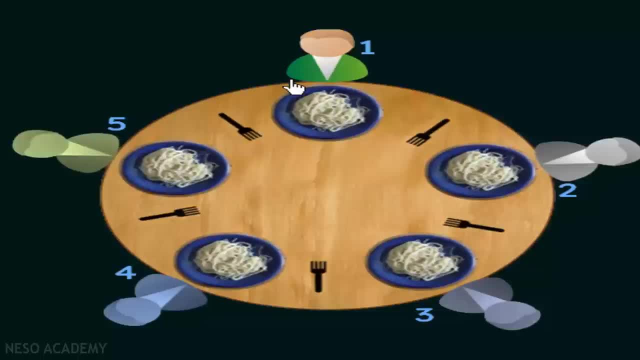 They have to pick up one and then the other. So let's say that all of them picked up the left chopsticks that were at their left. So, philosopher one will pick up his left chopstick, which is this one. Two will pick up his left chopstick. 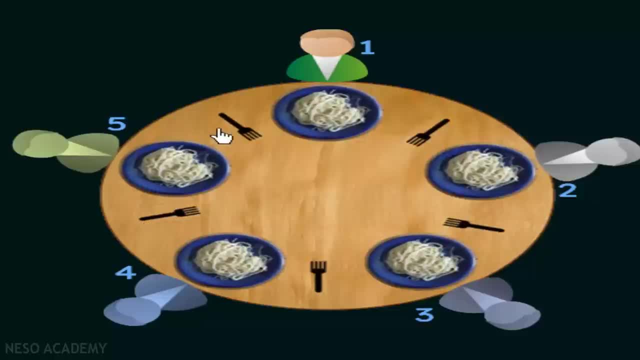 which is this one, Three will pick up this, Four will pick up this and five will pick up this. Now, if you see, all the chopsticks are picked up by one of the philosophers. Now, let's say, one is trying to eat. 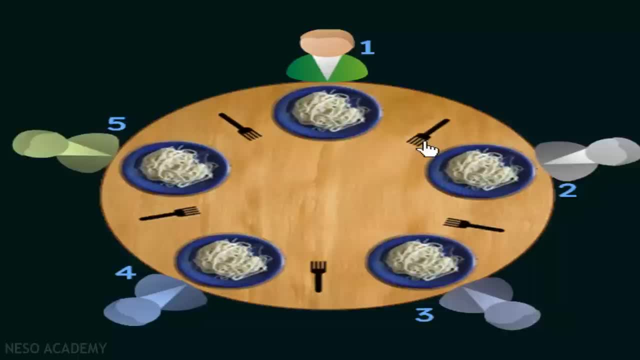 So what will he do? He have already got one of the chopstick. Now he needs a second chopstick to start eating. Which is the second chopstick? It is this one, But can he get it? No, because five is holding it. Similarly, 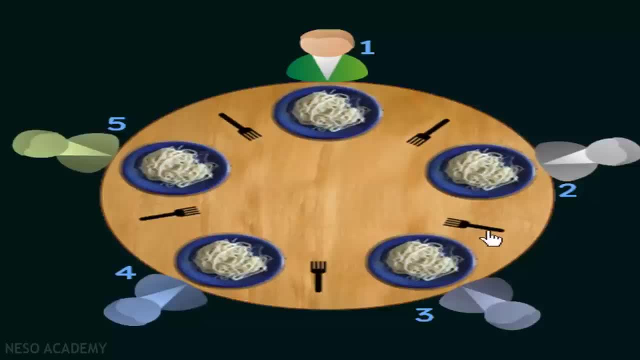 two has got hold of this chopstick, which is at his left. Now for starting to eat, he also needs the chopstick that is at his right, which is this one, But it is being held by one. It is not able to eat it. Similarly, 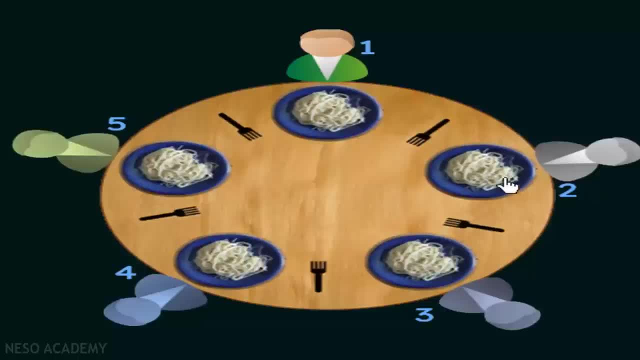 three also will not be able to get the right one because it is held by two. Four also will not be able to get this because it is held by three, And five also will not be able to get because it is held by four. So, according to, 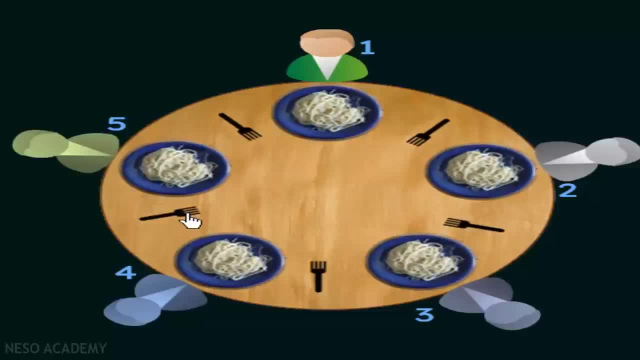 this problem: when a philosopher has one of the chopstick, he also needs the other one and he will keep waiting for getting the other one to start eating. But you see here that each of them are waiting for each other And nobody is going to release it. 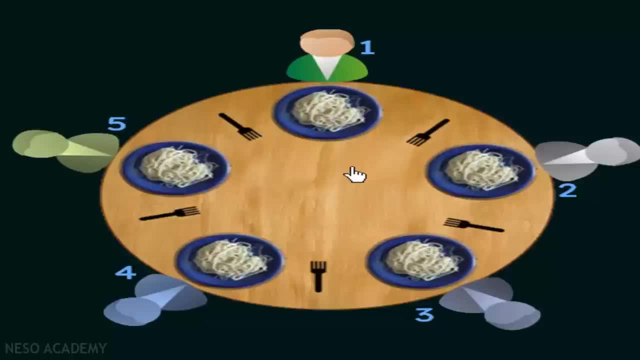 because all of them wants to eat And they all have one chopstick each. So each of them, they will be waiting for each other and they will keep waiting here and nobody is going to release it. So at this situation, we say that we have. 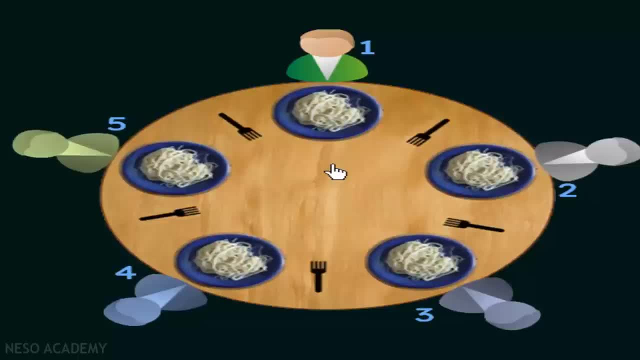 reached a deadlock, So this scenario is known as a deathlock. So this kind of same situation can even happen with resources that are shared among processes in our operating system. So this is something that we have to avoid. So that is what we have. 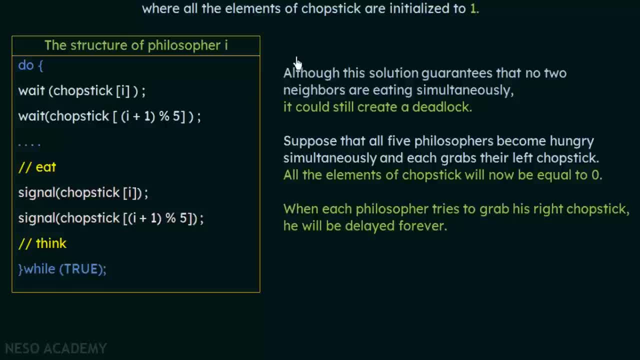 just said here. So that is the problem that we are going to face here. We have solved one problem, which is: no two philosophers adjacent to each other should start eating at the same time. We have solved that using the semaphores here. 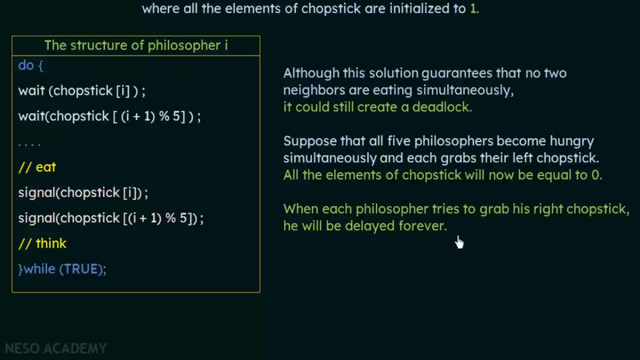 But still this problem persists, which could lead to a deathlock. So now we have to find if there are any ways that we can propose in which we can avoid this deathlock. So let's see if there are any remedies that we can follow in order to avoid. 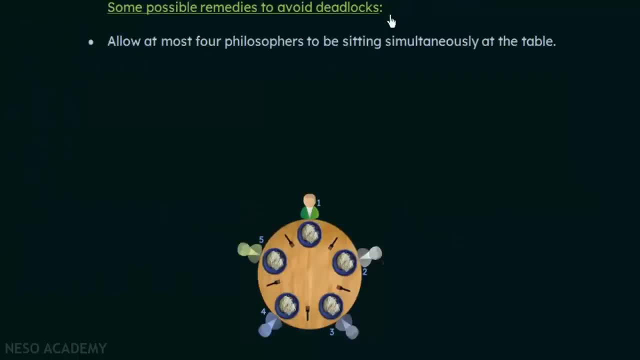 this deathlock. So here we will be discussing some of the possible remedies to avoid the deathlock. So the first one is allow at most four philosophers to be sitting simultaneously at the table. So here, instead of allowing five of them to sit, we would be allowing 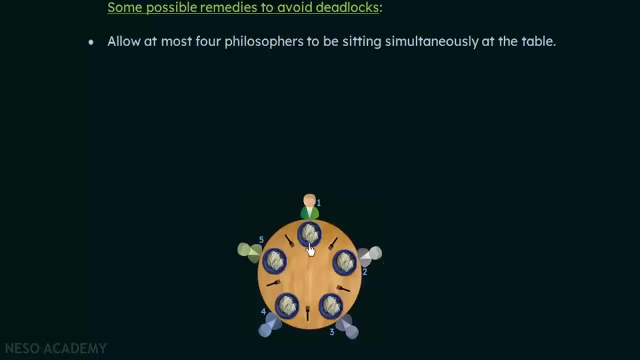 only four of them to sit simultaneously at the table. So the number of forks will remain the same, but the philosophers will only be four here. So what will happen? Even if all of them get hungry at the same time and pick up, let's say, the left forks, what will happen? 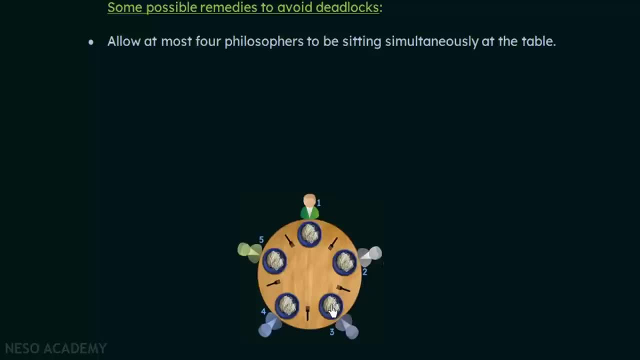 Philosopher. one will pick up this, two will pick up this, three will pick up this and four will pick up this one. So we assume there is no five now. So we see that one fork is still free over here. So 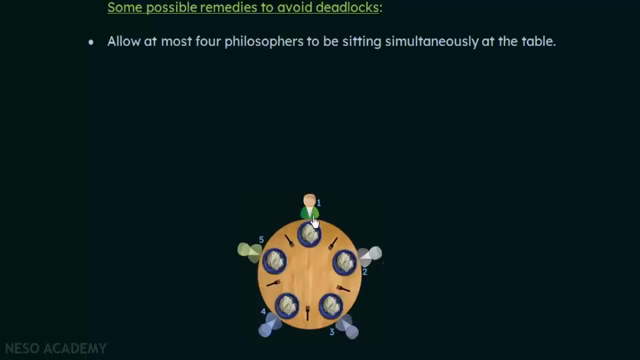 what will happen, Philosopher? one will pick this up and he will start eating, and then, after he finishes, he will keep it down. and when he keeps it down, two will get hold of this and he will also start eating and after he finishes, he will. 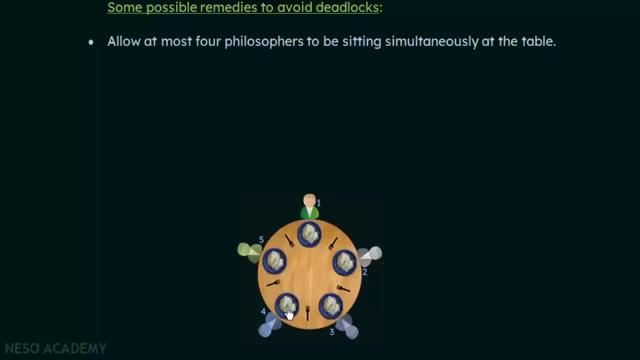 keep it down and three will get his chance and four will also get his chance. So we see that if we avoid one of them, then we can avoid the deadlock situation. So that is one possible remedy that we can have to avoid the deadlock. 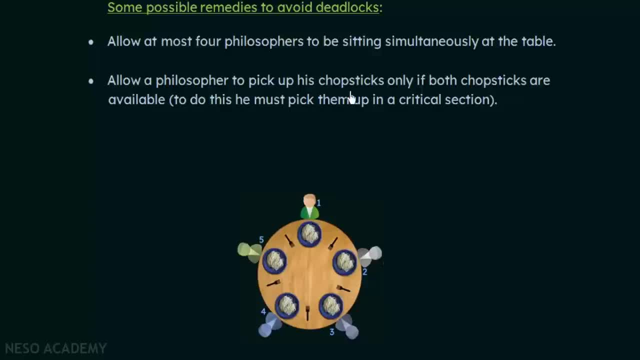 Then the second remedy is: allow a philosopher to pick up his chopsticks only if both chopsticks are available To do this. he must pick them up in a critical section. So here we saw that in the first scenario, when all of them got hungry. 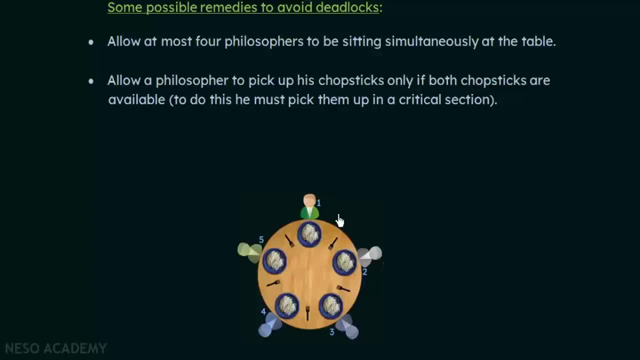 at the same time, they just picked up the fork that was available and did not see if the other fork is available or not. So, instead of doing that, we will allow the philosophers to pick up their chopsticks only after making sure that both the chopsticks that they 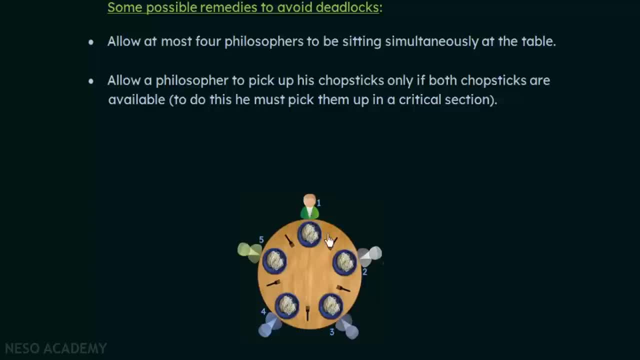 need are available. So if one wants to eat, he will make sure that both this and this chopsticks are available, and then only he will pick up one by one. So that is another solution that we can have in order to avoid this.